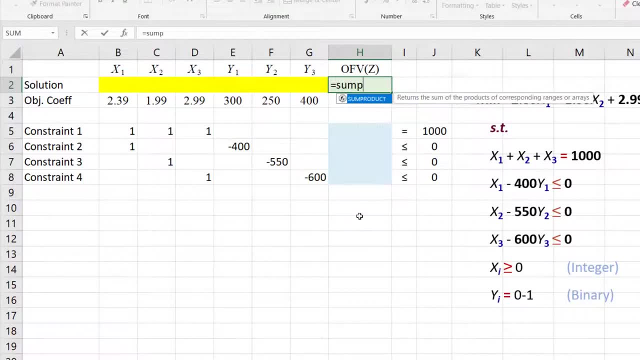 formula in this green cell by using equal SUMPRODUCT. Highlight the coefficients Comma, Then the variable values in yellow here. That multiplies each coefficient with the adjacent variable and adds the products, Then enter. We do the same for the constraints. 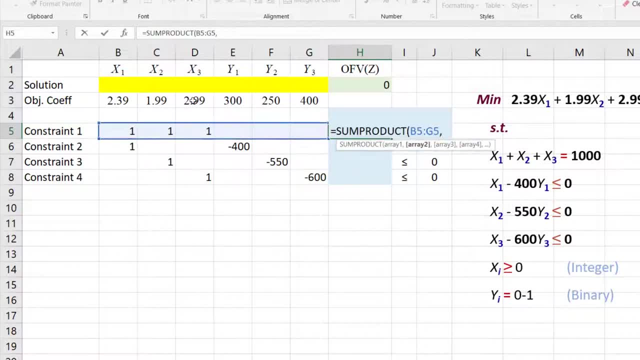 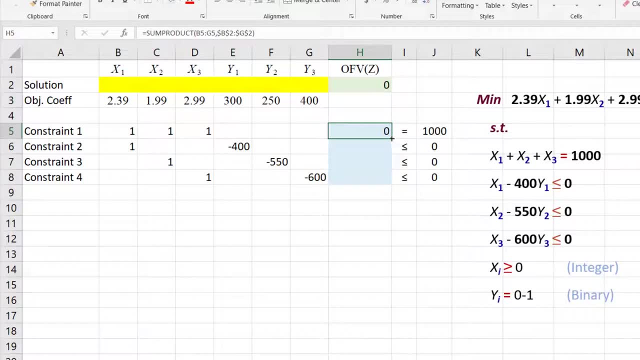 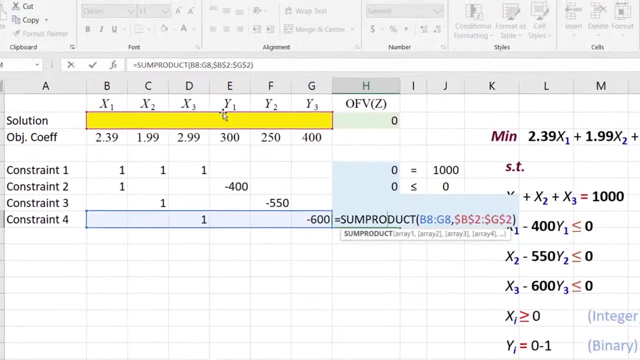 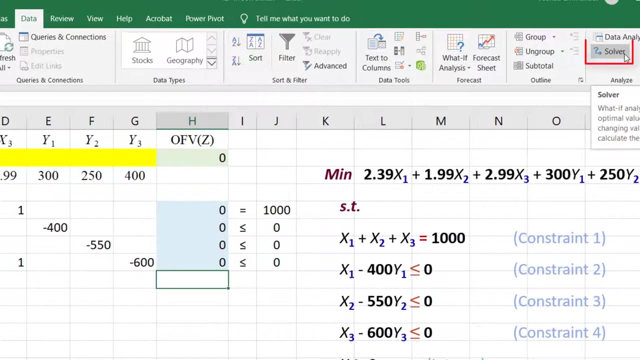 So I can drag to fill the other cells with the formula While keeping the yellow cells locked down. Double clicking the formula for the last constraint here shows that it worked. Now I'm going to click DATA, then SOLVER, to solve the problem. If you don't see SOLVER here, please see. 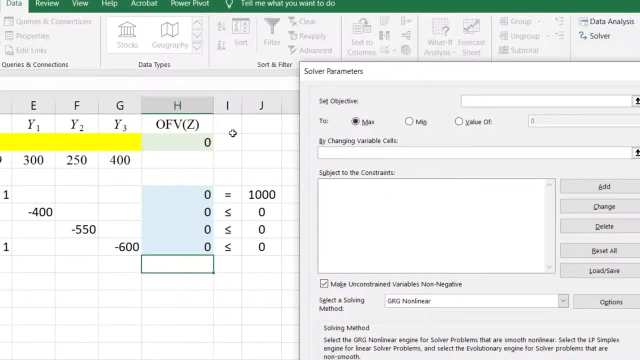 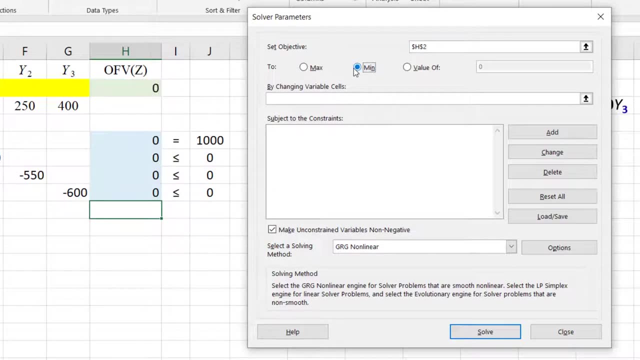 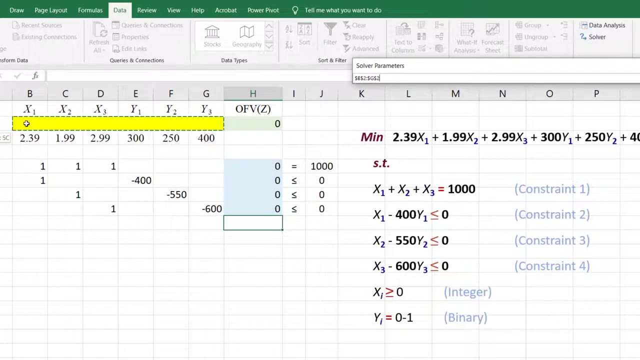 description on how to add it. For Set Objective: we will click the green cell that contains the objective function formula. here, Since this is a minimization problem, we will select Mean. here The changing cells will be the yellow cells that will contain the variable values at optimal. 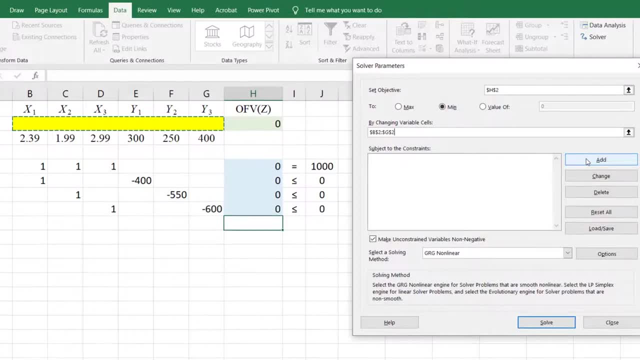 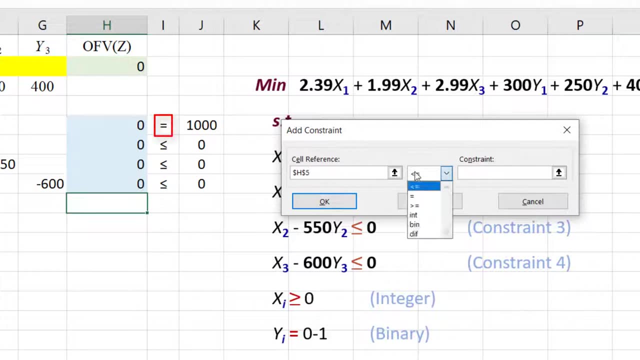 solution. Next click Add. to add the constraints, Click on the formula for the first constraint, select the equal sign. then click on the right hand side, Click Add. Since the remaining constraints all have less than or equal signs, highlight them all at. 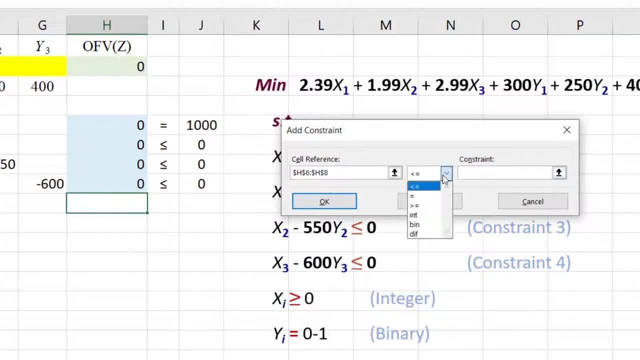 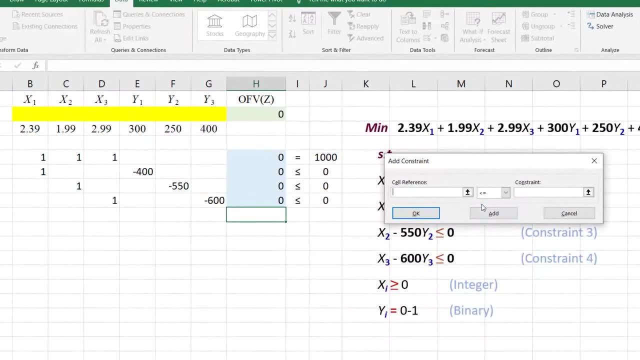 once, Select the less than or equal sign and then the right hand sides: Click Add. Since the Xs are integers, highlight their values here and select int for integer: Click Add. The Ys are 0,1 variables, so select them and choose Binary.